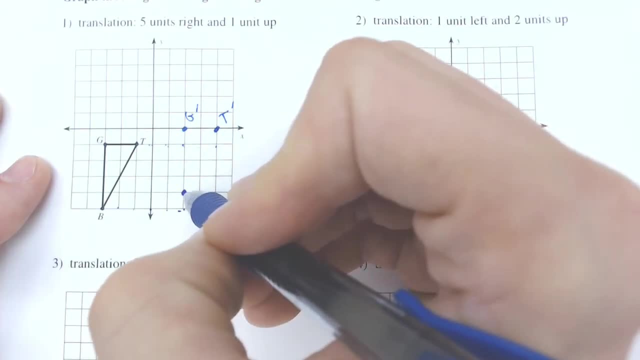 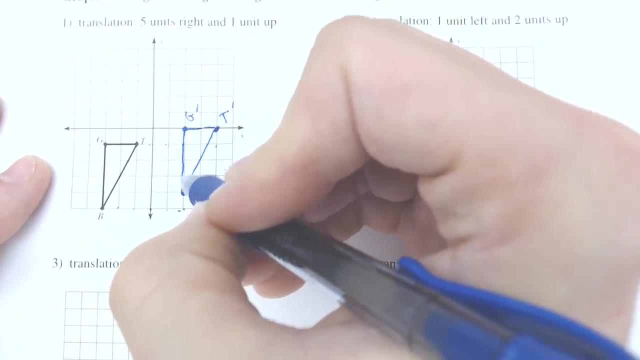 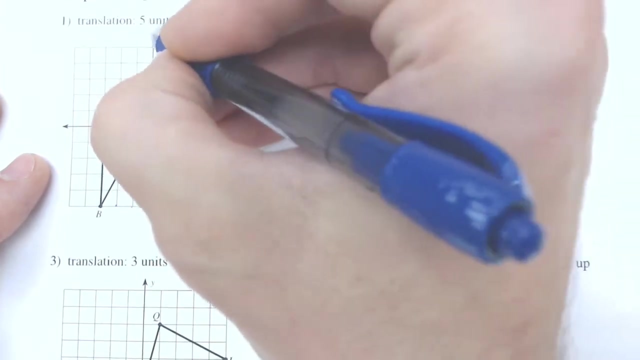 five, Four, five and one unit up, and if you have done it correctly, the shape that you make should be identical in every way. It's just move to the right and up by one. So the rule for this can be written a few different ways. They've written one way, but you could also write the rule as: 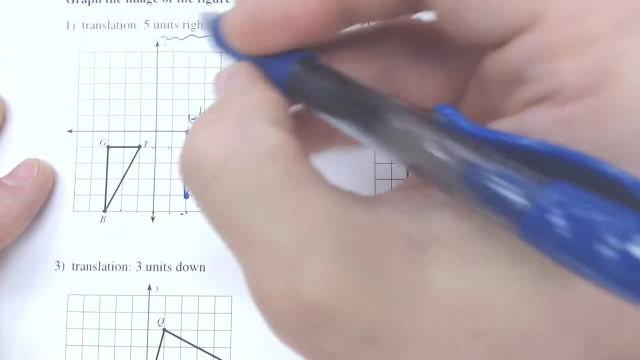 x plus five, because x is positive, like left and right numbers, and we went five units to the right, which meant it got bigger. So we're going to do that, So we're going to do that, So we're going to dropped two. So if we take что is lower than all of the values by 1,. 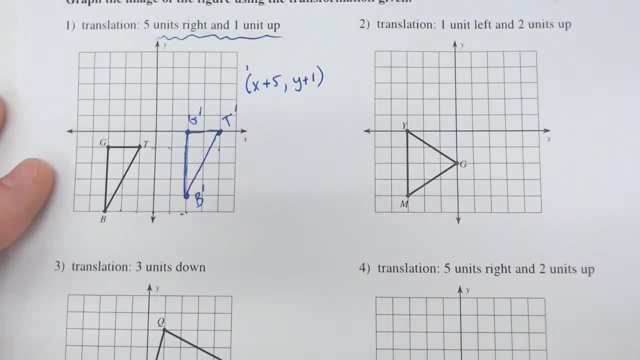 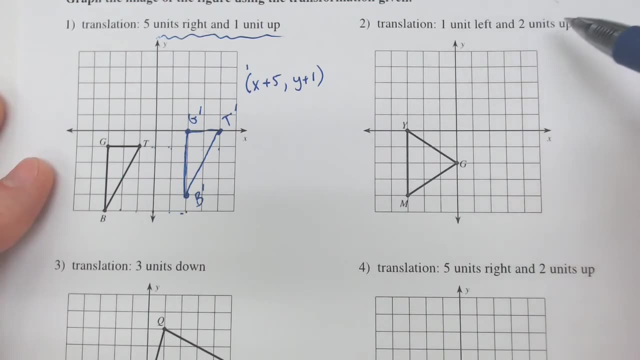 and y plus 1, and it's up to the left by one unit and up by two units. all of the x values are going to go to the left by one. So the x values will be subtracted by 1 and the y values will be increased by 2. so 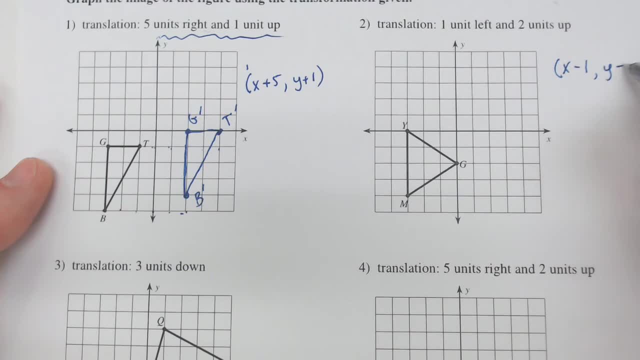 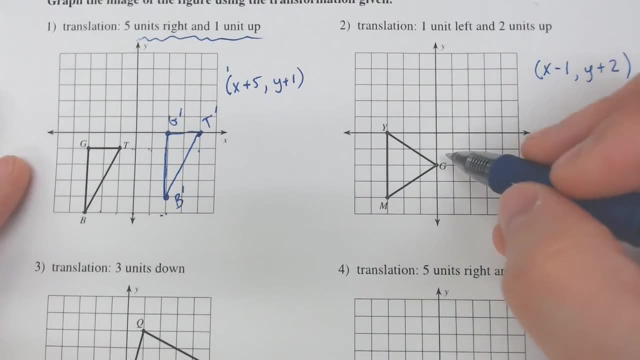 that would be a y plus 2.. So if we were only concerned with y, we obviously wouldicatted by one or an inverse of a, y, the actual coordinate values. Let's say that this value, right here, g, currently is at. 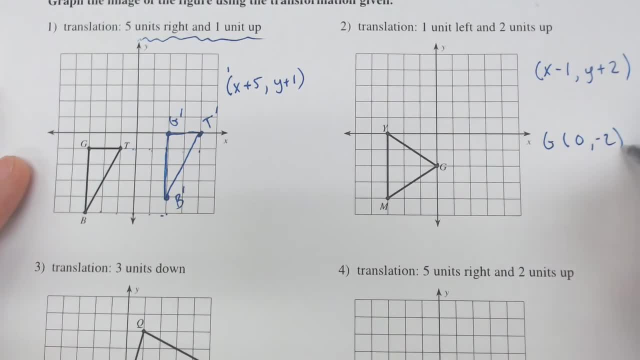 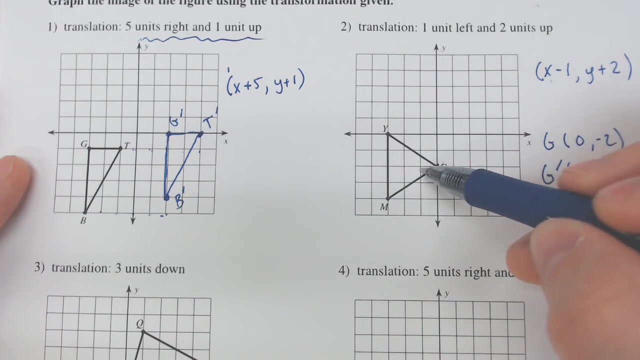 0, negative 2.. My new g prime is going to be subtracting 1 from 0,, that's negative 1, and adding 2 to negative 2, which makes 0. So really, when we go to the left by 1 and 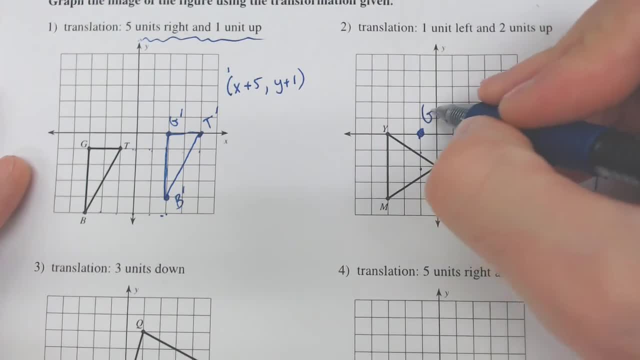 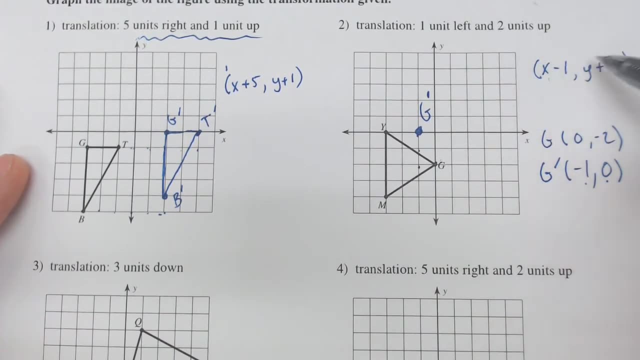 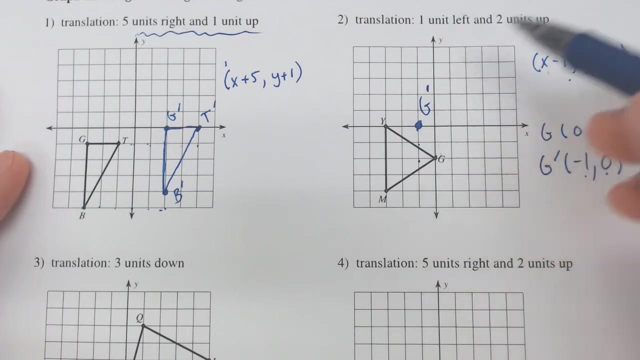 up by 2,. my g prime is right here, which is at negative 1, 0.. So you don't have to do that. but if you only are given coordinates, this is kind of useful to just subtract 1 and add 2, rather than actually graphing the entire thing. So I'm just going to plot the 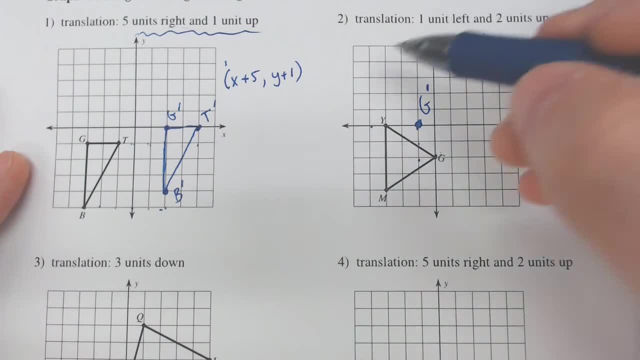 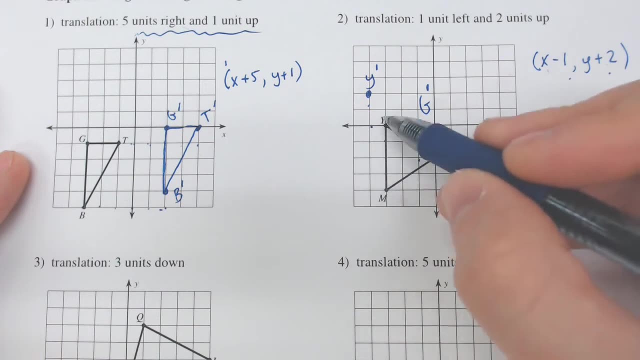 rest of them real quick. We got y has to go to the left by 1, and up by 2.. And I know that m is 1,, 2,, 3,, 4 units below y, so I'm just going to go 1,, 2,, 3,, 4 units below y. 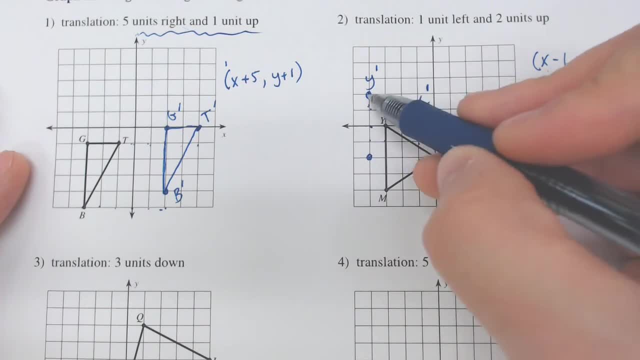 1,, 2,, 3,, 4 units below y. so I'm just going to go 1,, 2,, 3,, 4 units below y. so I'm just two, three, four units below Y to make that perfect, congruent shape and there 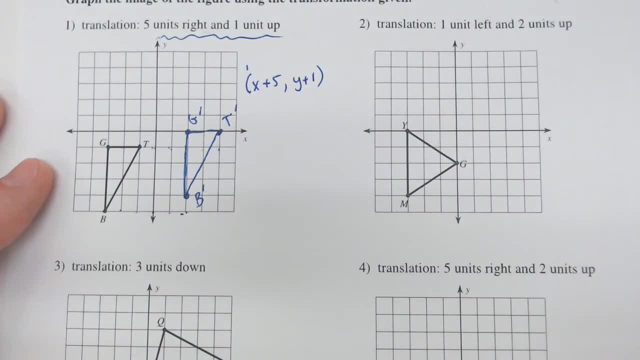 but we're just going to go with that, but you might want to do that, And so on. So we're going to do the same thing on the right and to the left, and then we're going to do the same thing on the right, which meant it got bigger and y plus one. 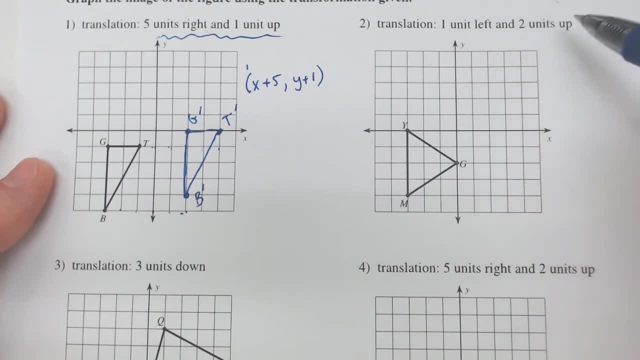 If we wanted to do this next one, which is to the left by one unit and up by two units, all of the x values are going to go to the left by one, so the x values will be subtracted by one and the y values would be increased by two, so that would be a y plus two. So if we were only concerned with 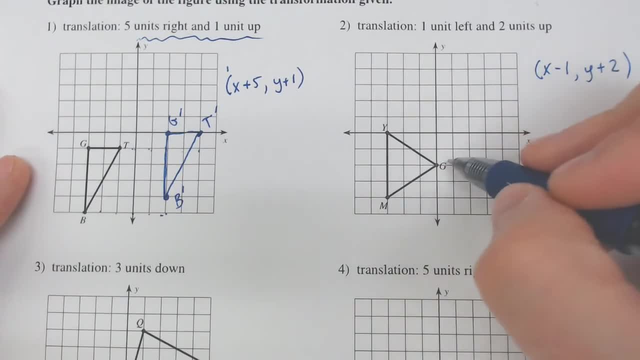 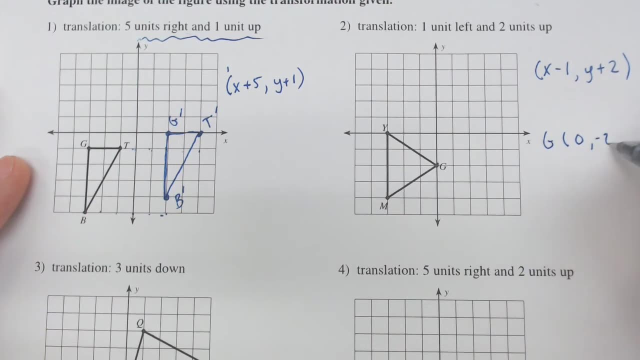 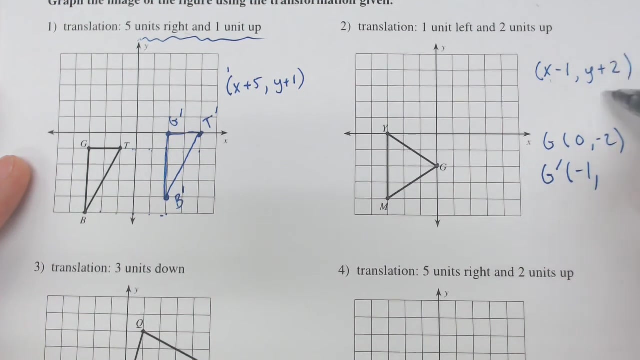 the actual coordinate values. Let's say that this value right here, g, currently is at 0, negative 2.. My new g prime is going to be subtracting 1 from 0,, that's negative 1, and adding 2 to negative 2, which makes 0. So really, when we go to the left by 1 and 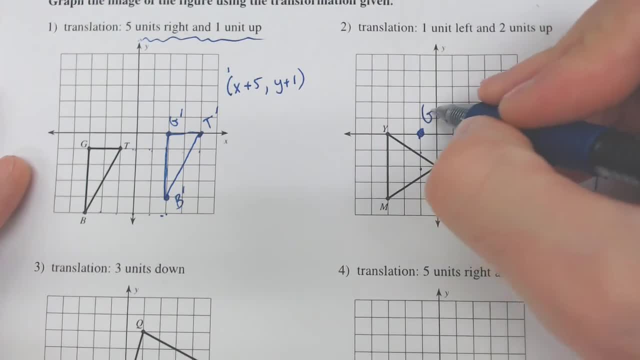 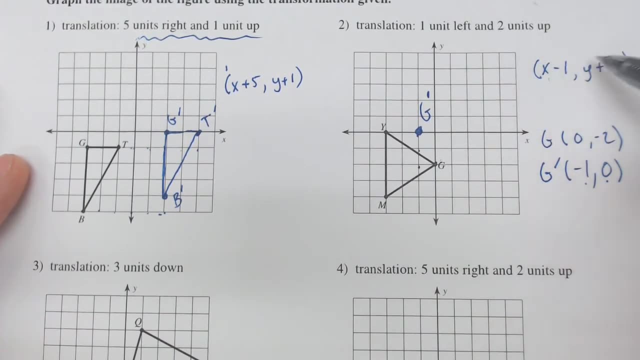 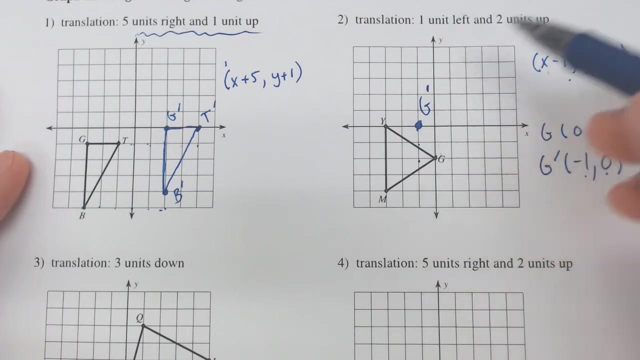 up by 2,. my g prime is right here, which is at negative 1, 0.. So you don't have to do that. but if you only are given coordinates, this is kind of useful to just subtract 1 and add 2, rather than actually graphing the entire thing. So I'm just going to plot the 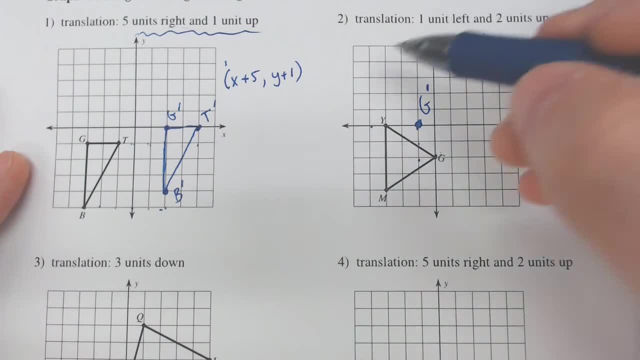 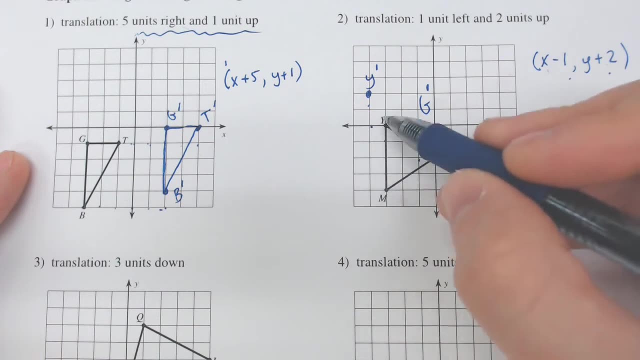 rest of them real quick. We got y has to go to the left by 1, and up by 2.. And I know that m is 1,, 2,, 3,, 4 units below y, so I'm just going to go 1,, 2,, 3,, 4 units below y. 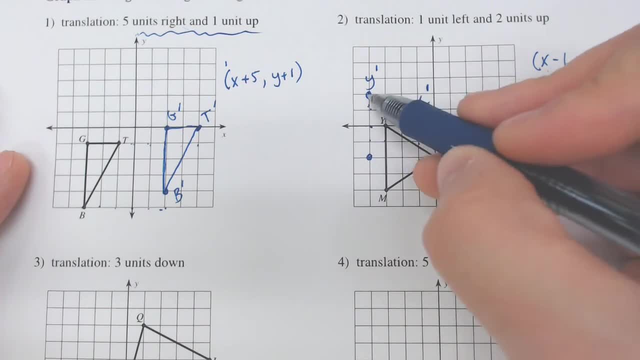 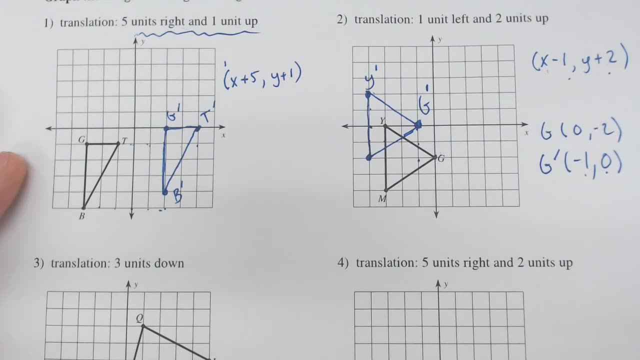 and up by 2.. So I'm just going to go 1,, 2,, 3,, 4 units below y. so I'm just going to go 1,, 2,, 3,, 4 units below y to make that perfect, congruent shape. And there we have it. So 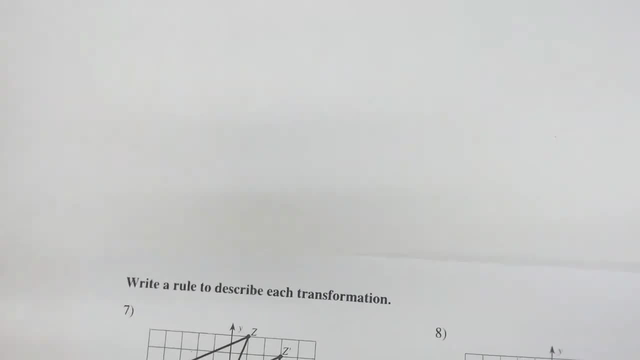 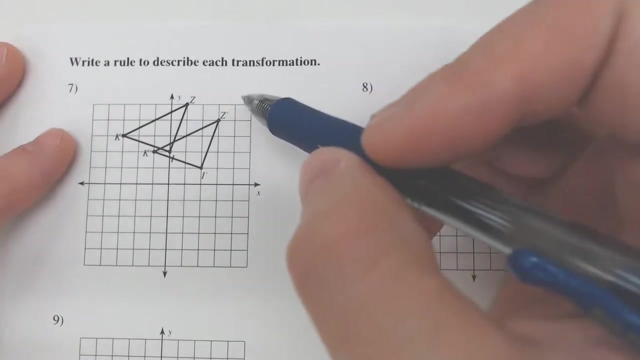 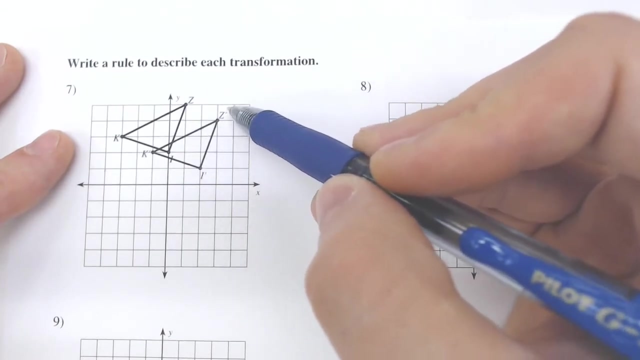 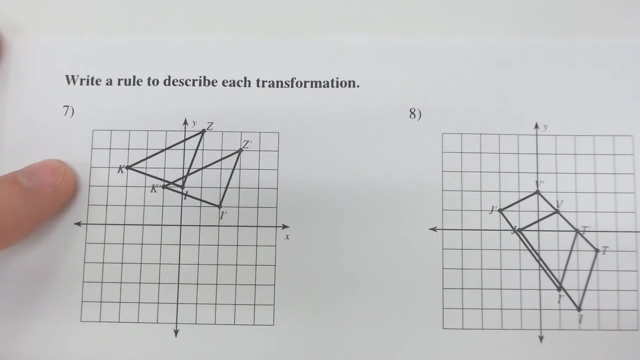 the next view that we're going to be doing is going to describe the rule. So write the rule that describes each transformation. You need to make sure that you're careful that you're not going to get lost. So we're going to go to the right by 1, 2, and down by 1.. 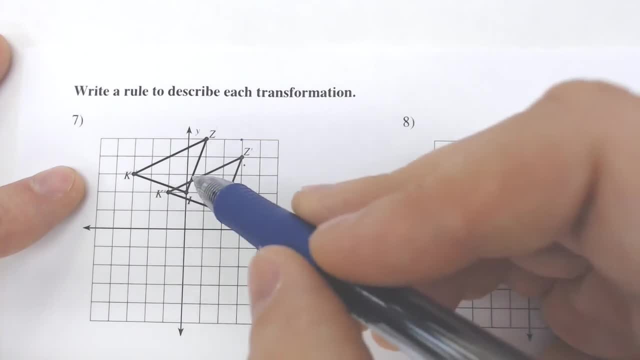 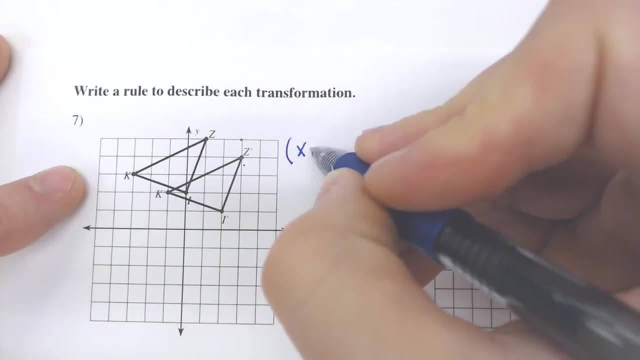 And all of these points are going to the right by 2 and down by 1.. So it doesn't matter which point you pick, They all went to the right by 2 and down by 1.. Well, x is to the left.